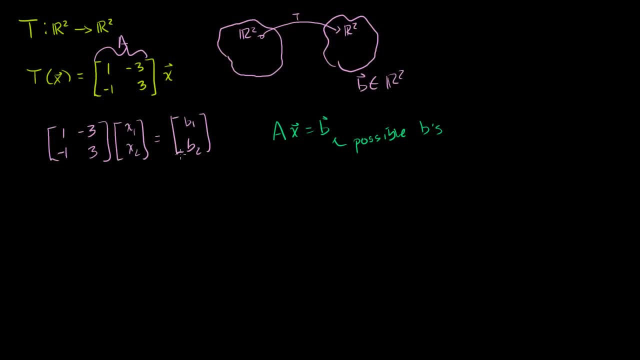 All of the possible b's. So if I were to solve this equation for any particular b, what I would do is I would put this in reduced row echelon form. Well, first I would make an augmented matrix of it, So I would put a 1,, a minus 3, a minus 1, and a 3.. 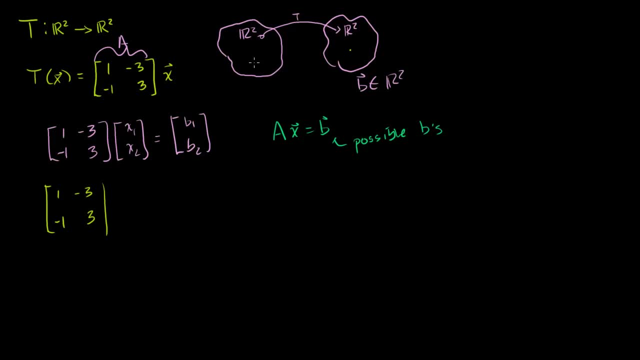 And I would augment it with the member of our co-domain. we're trying to be equal to, So b1, b2.. And then I would put in reduced row echelon form. So how can we do that? How can we put in reduced row echelon form? 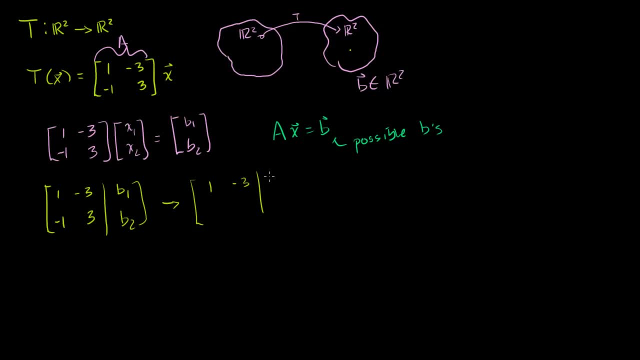 I'll keep my first row, the same: 1, minus 3, and then b1.. And then my second row. I'll replace it with my second row plus my first row. So minus 1 plus 1 is 0.. 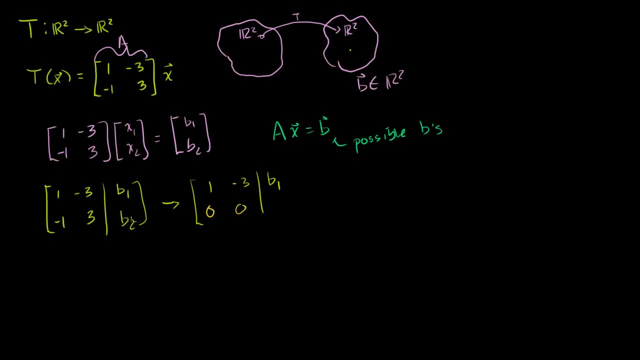 3 plus minus 3 is 0. And then b2 plus b1 is well, I could just write that as b1 plus b2.. So this is only going to have solutions. I have an interesting situation here. We've seen it before. 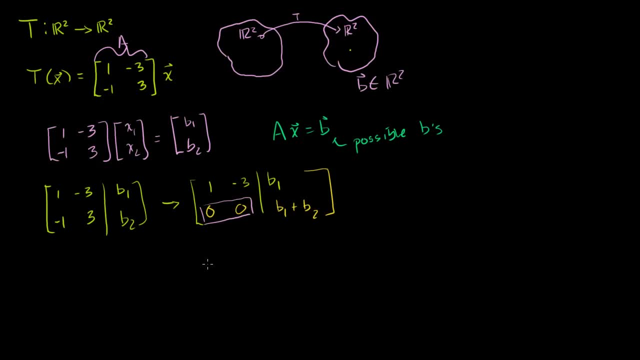 I have a row of 0's And the only way that this is going to actually have solutions is if this thing right here is also going to be equal to 0.. So the only members b that are members of Rm that have solutions are the ones where, if you add up their two terms, 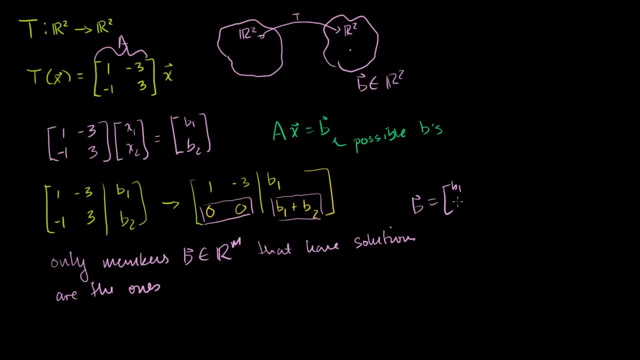 so let's say b is equal to b1 and b2, are the ones where the two terms are equal. The two terms added up have to be equal to 0. b1 plus b2 have to be equal to 0. Or another way you could write it is that b2 has to be equal. 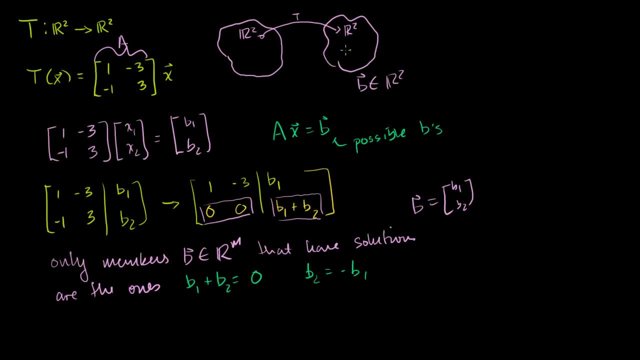 to minus b1.. So if we would actually draw our codomain, let's do it. We always stay in the abstract, but sometimes it's useful to draw an actual example. So let's say that our codomain is R2.. Let me draw some axes right here. 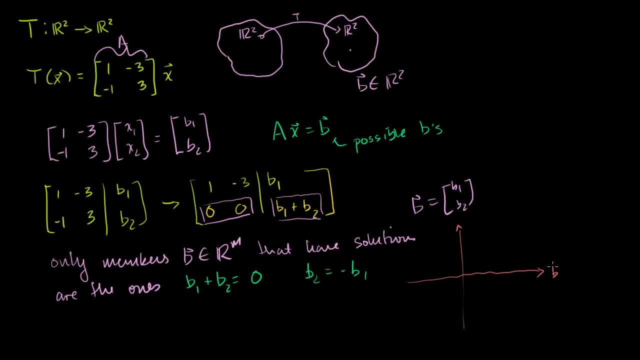 Let's say that this is my b1 axis And this is my b2 axis. I could have called that x and y, but I call that b1 and b2.. What are all of the members of my codomain that have a? 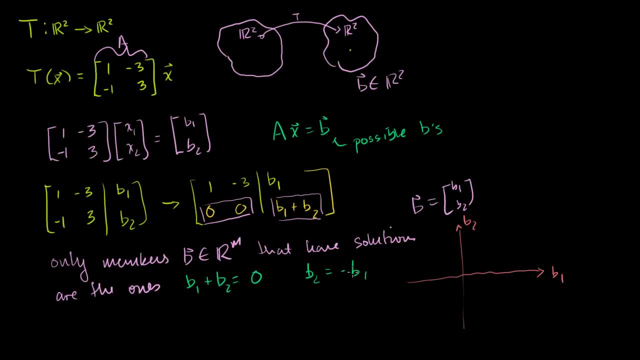 solution that have a mapping. Well, b2 has to be equal to minus b1. So it's going to look like this. Let me draw this. It's going to be aligned with a slope of negative 1.. This is all the b's that have solution. 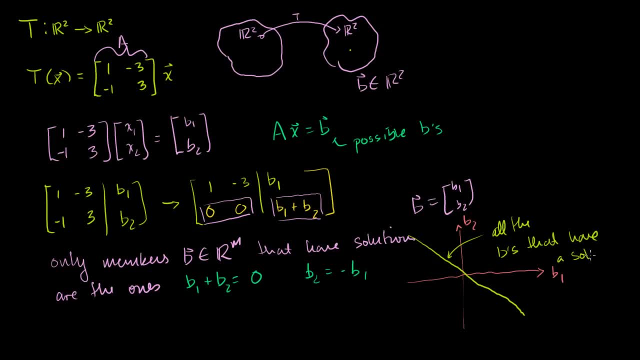 That have a solution, Because if you're not on this line, if you're a member of your codomain, this is the codomain right here: R2.. R2 is also our domain, but let me make it very clear that this is the codomain that I've drawn. 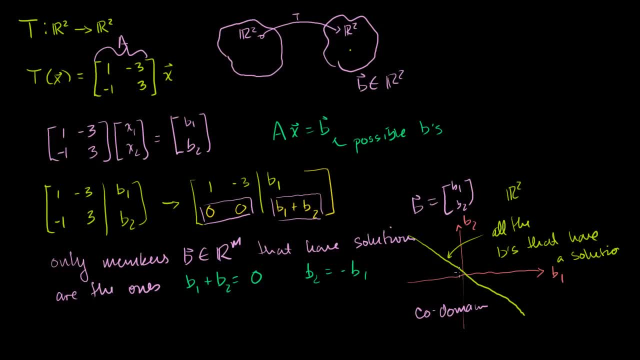 This is what we're mapping into. It's very clear that if we're not on this line, if you pick somebody whose two terms don't add up to equaling 0 or aren't the negative of each other, if you pick someone over here in, 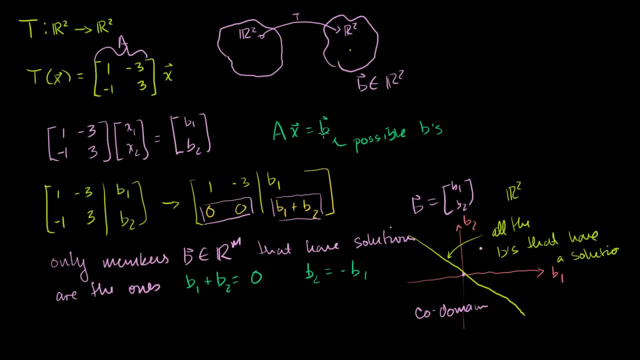 our codomain, and then you try to solve the equation over here. you're going to have a 0 is going to equal some non-zero number here and you're not going to have a solution. We touched on this in the last video. 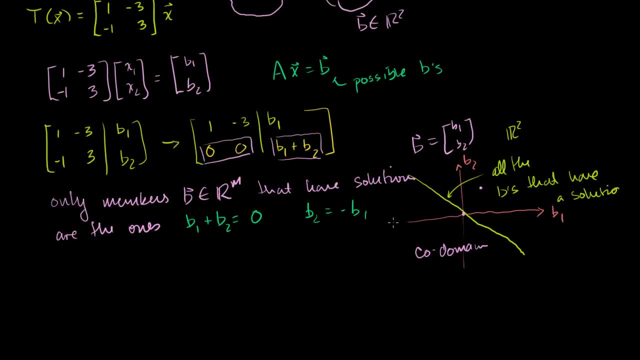 So, in this case, the image. we could say that this right here is the image of our transformation, or even another way of thinking about it. Obviously, if all of R2 is equal to 0, then you're going to have a solution. 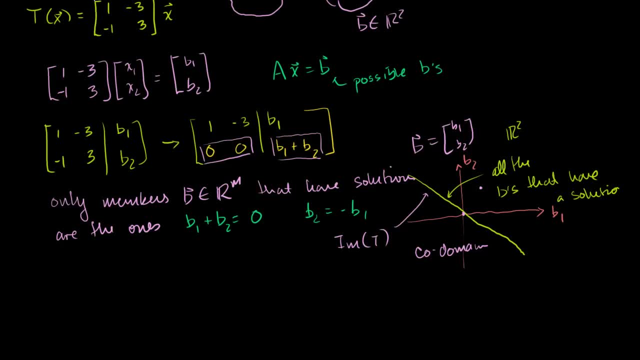 This is our codomain. Let me draw a domain. If our domain looks like this, if all of R2, so if you take any member of R2 and it's always mapping onto something onto that line, clearly each point on that line is going to. 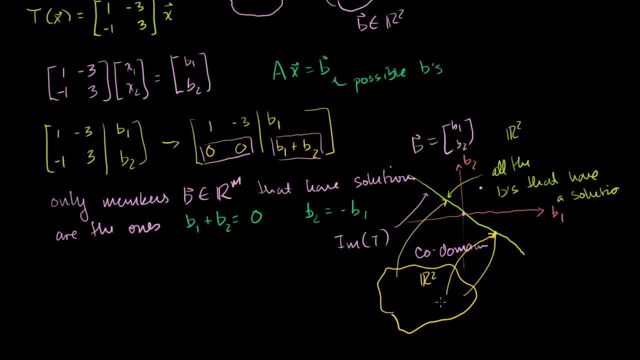 be mapped to by more than one vector. So we're not dealing with an onto transformation, And we saw that in the last video. In order for something to be onto, when you put it in reduced row echelon form, you cannot have all zeros in one of the rows. 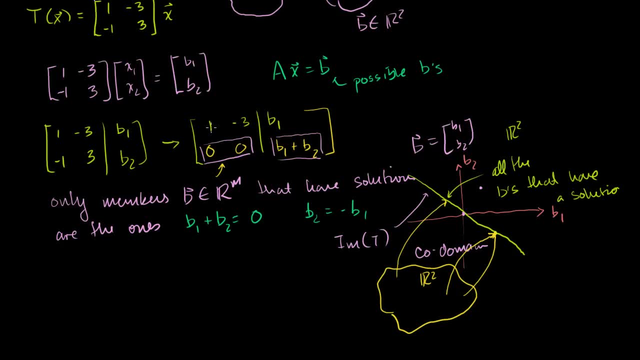 Or another way to say it, in reduced row echelon form. every row has to have a pivot entry, But let's focus on the b's that actually do have a solution. So let's focus on these b's so that when you take a b1 plus, 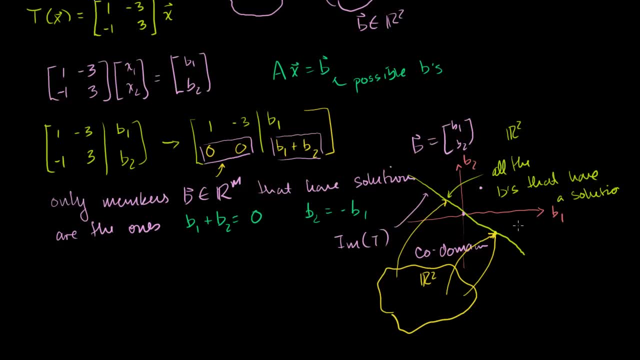 b2, it actually is going to be equal to 0. So we could have the b- I don't know. that could be the b5 minus 5, or you could have the b. well, obviously the b00 is going to work. 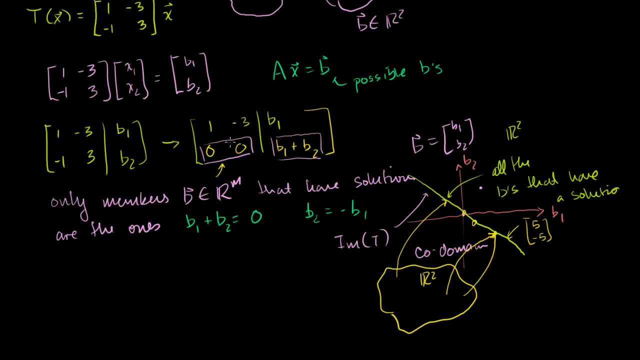 You could have 1, negative 1.. Maybe that's right there. Let's focus on those for a second and solve and see how many guys, how many members of our domain, map into them. So if we take this right here and then we apply this, 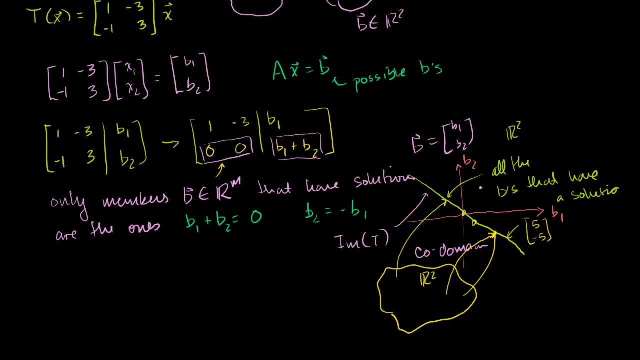 equation up here we only have one constraint. We're assuming that this is going to be equal to 0.. So let's assume that we're dealing with b's in our image. So let's assume that we're dealing with something where we can get a solution that b1 plus b2 is equal to 0.. 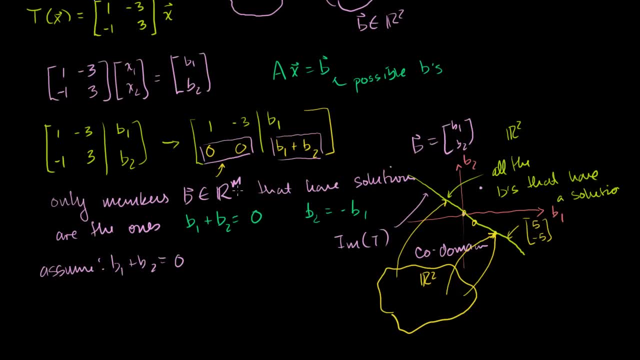 Then what is our constraints? What will map to our vector b that we're dealing with? So if we just take this top equation right here, we have 1 times x1, 1 times x1, let me switch colors. We have 1 times x1 minus 3 times x2 is equal to b1, and 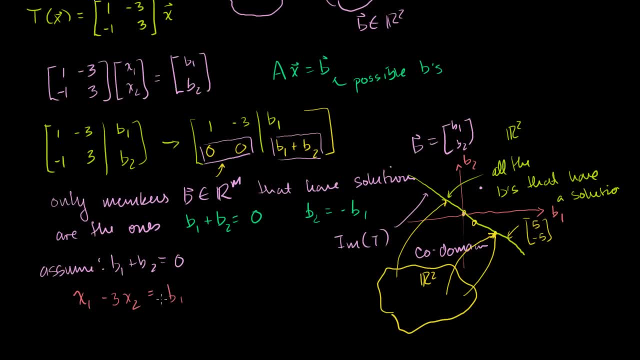 then this row will give us a number. There's no constraints because this is just going to be a bunch of 0's, So this is the only constraint for a member of our domain that will map to some particular b now that we are picking some. 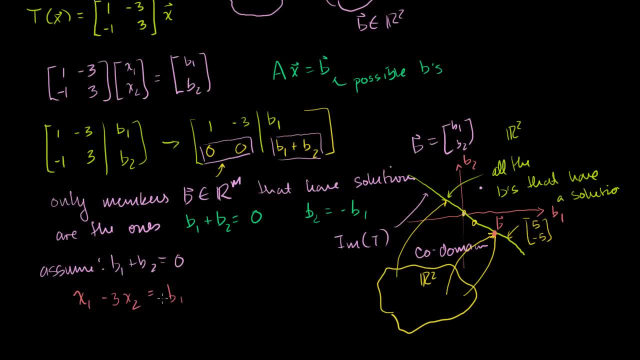 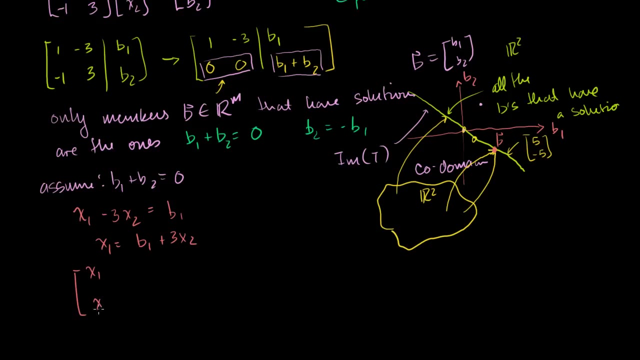 particular b that satisfies this constraint. So we could write this solution set. let me rewrite it as: x1 is equal to b1 plus 3x2.. Or if we wanted to write the entire solution set, it would look like this: x1, x2.. 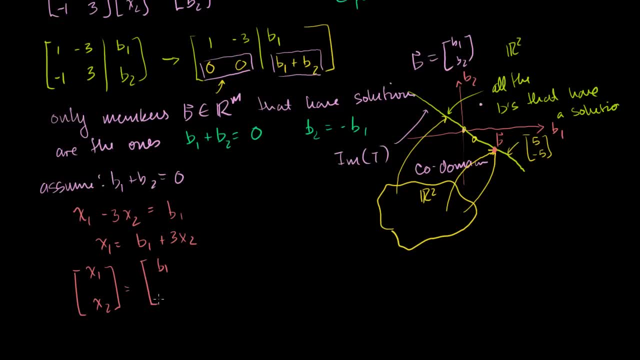 x1 is equal to the vector b1, 0, plus let's see x2.. x1 is b1 plus 3 times x2.. So plus x2 times 3.. And x2 is just going to be equal to x2.. 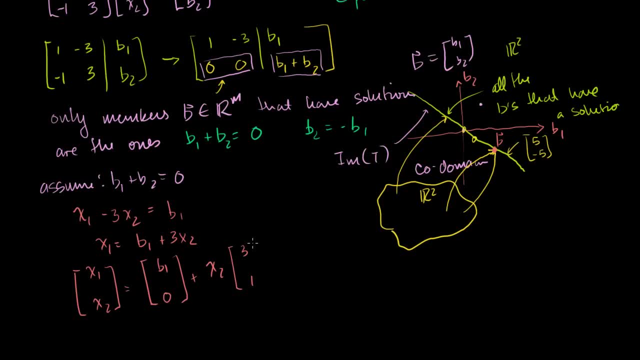 That's a free variable, So x2 is equal to 0 plus x2 times 1.. So what we're saying here is: look, this transformation just maps to this line here for all of the vectors in our codomain Where their two entries add up to each other. 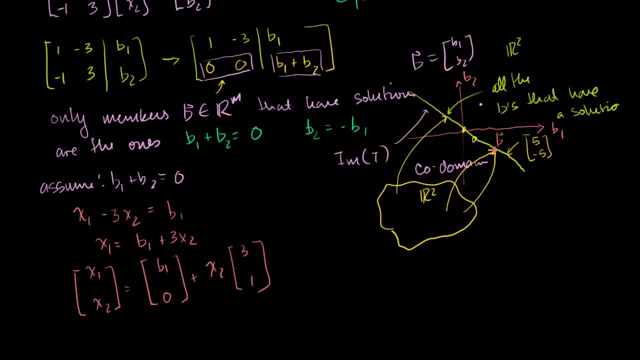 Now, assuming, let's assume that we actually have one of those vectors And so, first of all, this is definitely not an onto transformation, But let's assume that we are dealing with one of those guys. So, if we are picking a particular one of those guys, 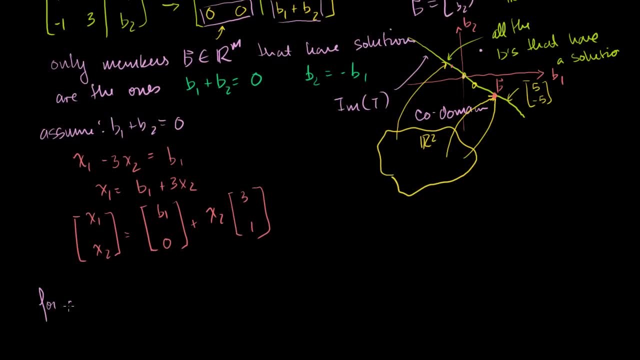 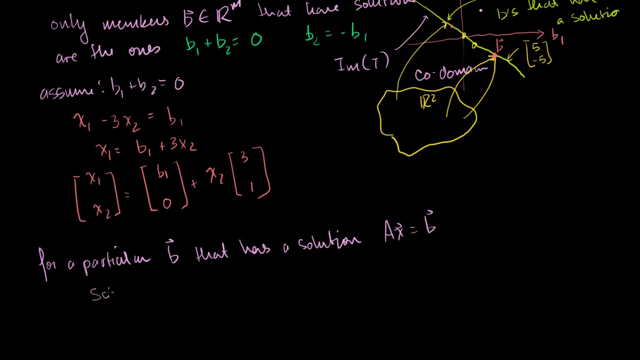 for a particular b. let me write this down: for a particular b that has a solution, that has a solution to Ax is equal to b, The solution set, the solution set, the solution set will be equal to this thing, right here. 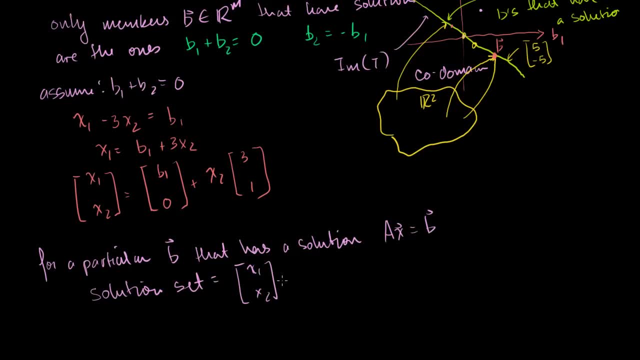 It will be equal to x1,. x2 is equal to the first entry of your b: b1, 0, plus x2 times the vector 3, 1.. And if you think about this, If you pick a particular b, 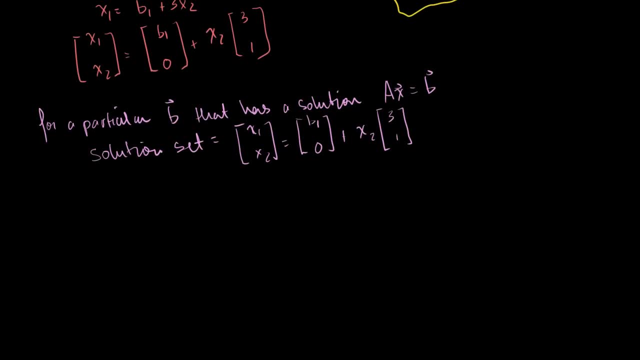 So let's say we pick our. let me draw this out because I think it's nice to visualize it all. Actually, maybe I'll draw it like this: I don't want to draw our blobs anymore, So let me draw my axes. 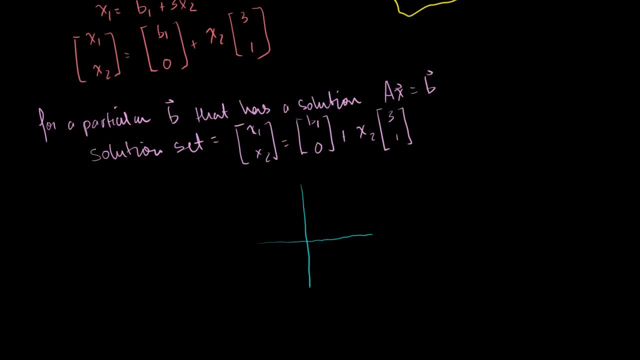 So my axes look like this: We know that the image of our transformation is aligned with a negative 1 slope, because the two entries have to be equal to the negative of each other. Let's pick a particular b. Let's pick a particular b that has a solution. 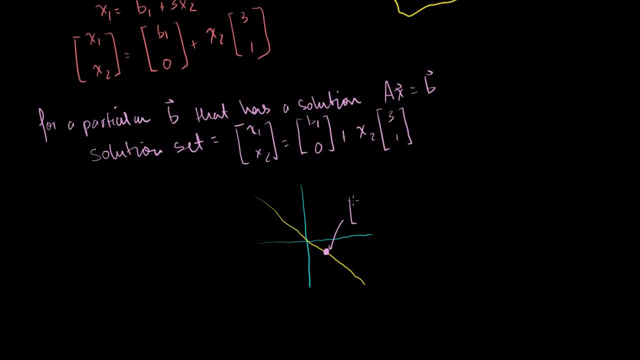 So let's say we pick That b right there. In order for it to have a solution, its entries have to be the negative of each other. So let's say that's the entry. Let's say that's the entry. 5 minus 5.. 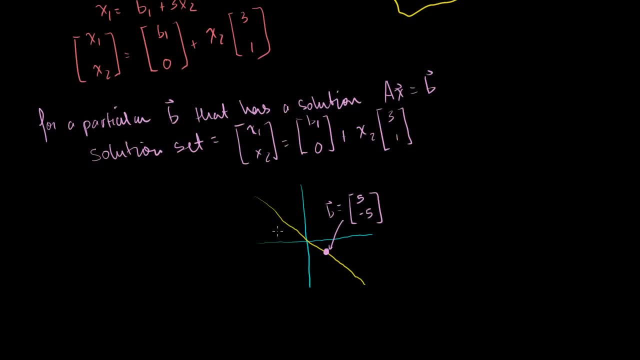 That is our b. So what we just showed is that the solution set if we want to say, hey, what in our domain maps to this guy? So let's think about what in our domain maps to this right here. Let's think about what in our domain maps to this point? 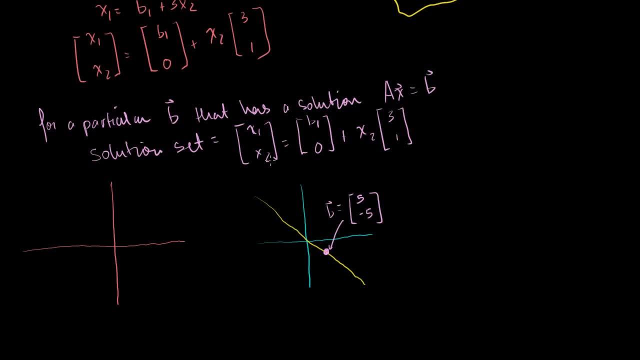 right here To this particular b, So that's going to be all of the x's that satisfy. ax is equal to 5 minus 5.. And what this is telling us is this is going to be equal to, so the solution set is going to be equal to. so x1, x2 is. 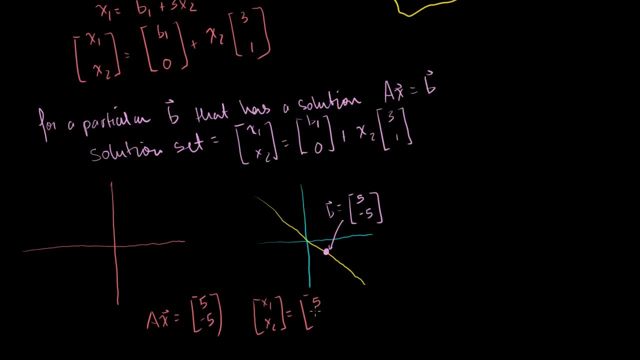 going to be equal to b1, is going to be equal to 5, 0, plus x2, plus any scalar multiple of the vector 3, 1, and 3, 1.. So our solution set is going to be: you take the vector 5, 0,, so 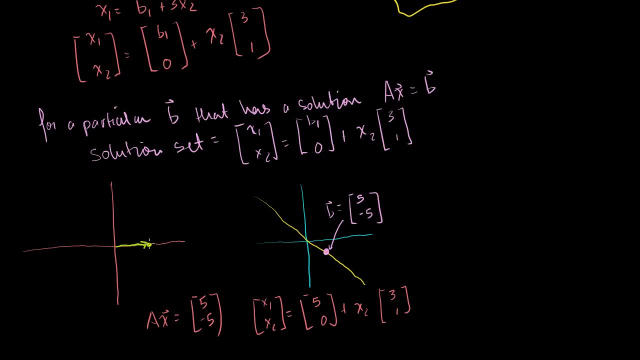 maybe the vector 5, 0 specifies this position right here, And then you're going to add to it multiples of the vector 3, 1.. The vector 3, 1 looks like this: 1,, 2,, 3, and you go up 1.. 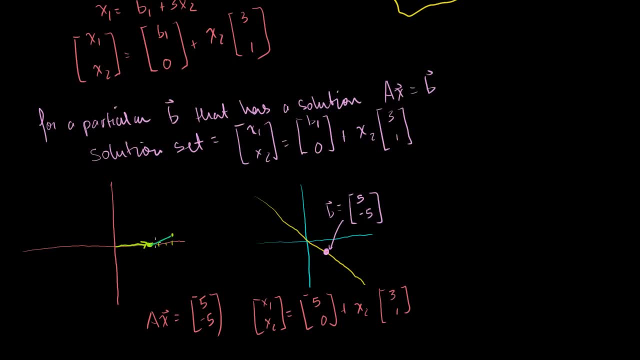 The vector 3, 1 is going to look like this: If you add multiples of this, multiples of that could stretch out like that or it could go negative like that to this vector 5, 0.. You're essentially going to. let me see if I can draw this. 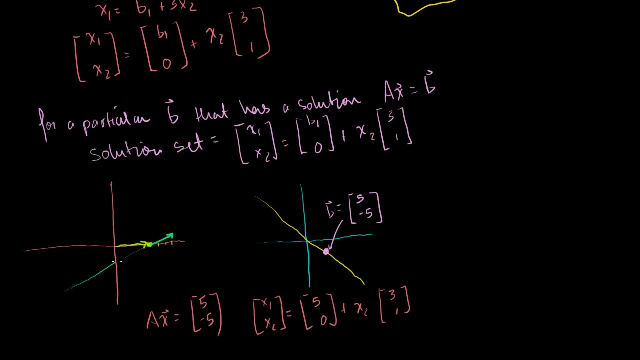 neatly, you're going to end up with a solution set that looks like that right there. So if you pick a particular B right there, that has a solution. we just said that everything on this line will map to that point in our solution set. 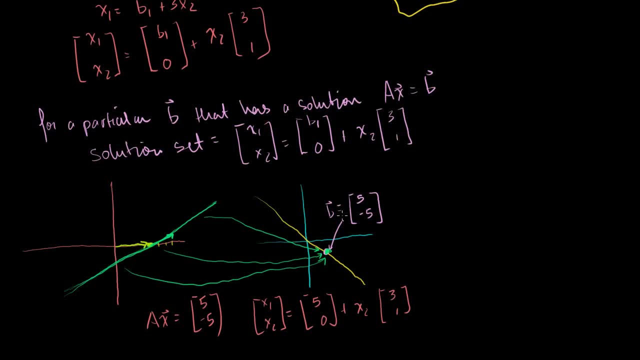 Everything on that line would map to our solution set. And in fact, if you picked another point- let's say you picked the point minus 5, 5,. let's say you picked- let me write it this way- minus 5, 5,. then the solution set that 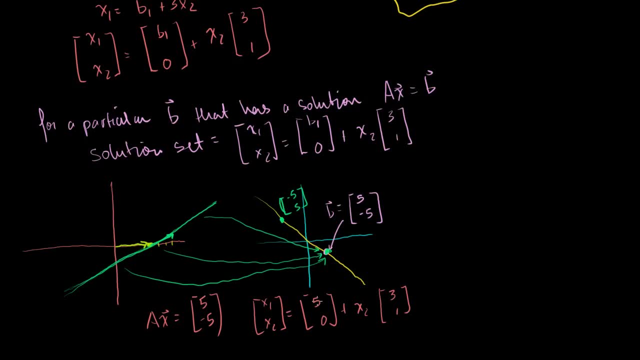 maps to that would actually be. you would take minus- this first term would be the minus 5, it would be here and all of these guys would map to that. Well, this is all interesting. I mean, we've been doing a lot of abstract things and I 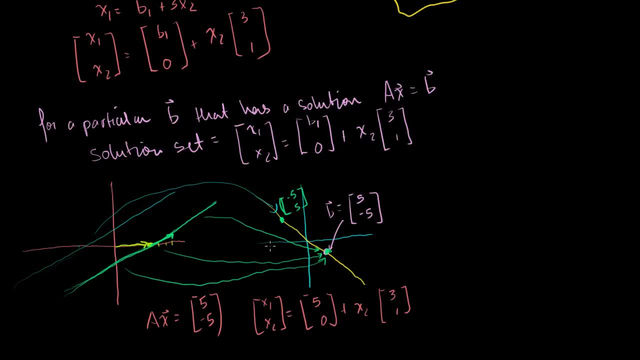 think it might be satisfying that you're actually seeing something kind of more concrete in this example, But I'm doing all of this for you. I'm doing all of this for a reason: because I want to understand what the solution set is to a general non. 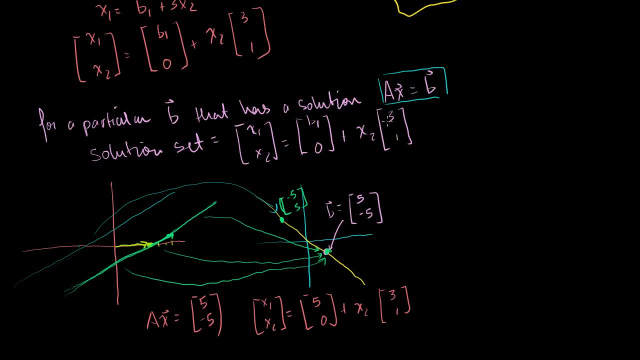 homogeneous equation like this And to understand a little bit better, let's imagine what is the solution set if I were to pick this guy, if I were to pick the 0 vector. If I pick the vector, this is the 0 vector, right there. 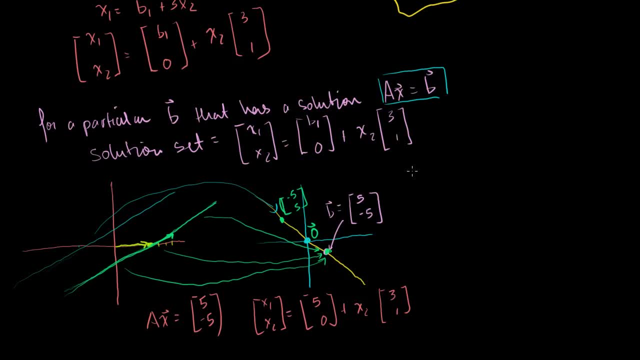 Then what's going to be the solution set? It's going to be the vector. so if we say that Ax is equal to 0, then our solution set is going to be the vector: 0, 0, plus right, 0, 0, plus x2 times 3, 1.. 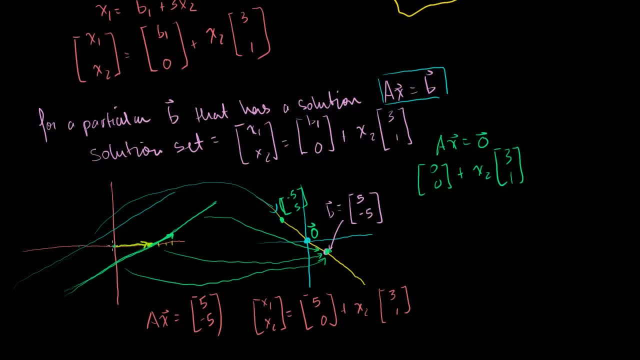 So it's going to be what It's going to be. this is just the 0 vector, so it's going to be here and it's going to just be multiples of 3, 1.. So it's going to look like. let me see it's going to look. 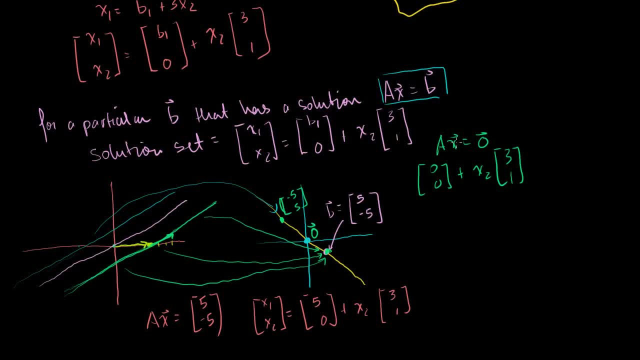 something like that. But what's this? What is the solution set to the equation of Ax equal to 0?? This is the null space. This, by definition, is the null space. This is the null space of A. This, right here, is the null space of A. 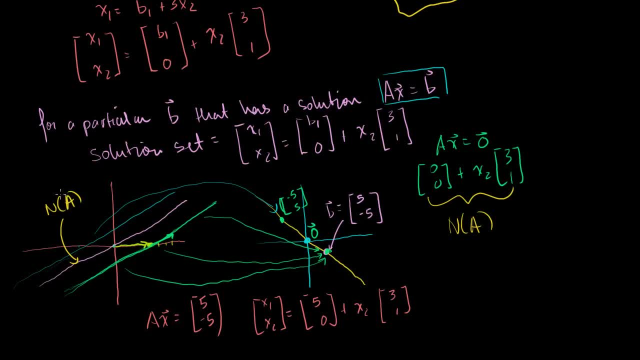 So notice- and this is the big kind of takeaway from this video- is that for any solution, we're picking B's that actually do have solutions. because we're picking them on this line, We're picking them in the image of our codomain. 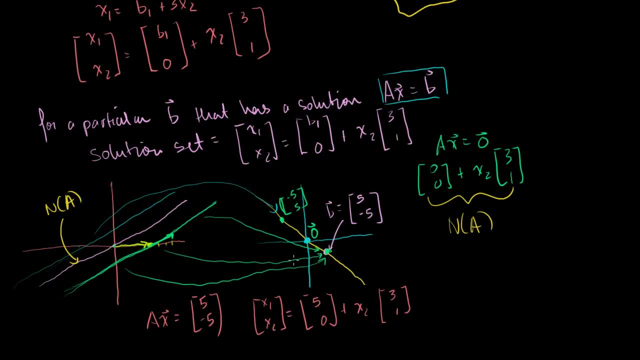 But the solution set to any Ax is equal to some B. where B does have a solution, it's essentially equal to a shifted version of the null set. This right here, or the null space. This right here is the null space. That right there is the null space for any real number x2.. 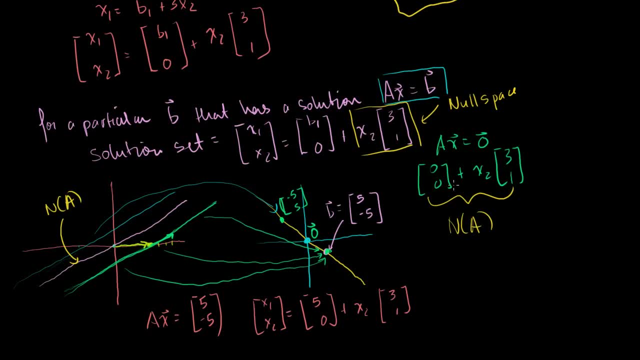 Any scalar multiple of 3, 1 is the null space. I just showed it right there. It's going to be that, And so all of these other solution sets are just some particular vector, some x particular plus the null space, plus the null space. 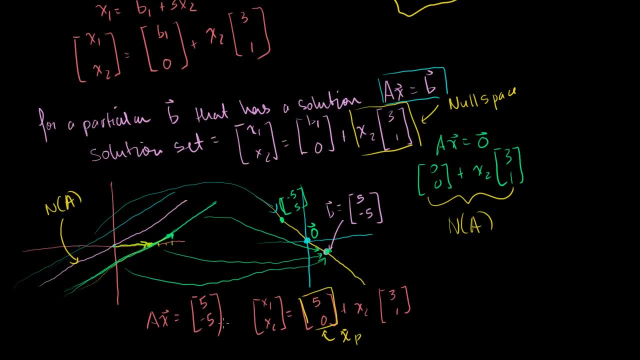 Obviously this vector by itself would also be a solution to Ax is equal to B, Because you could just set x2 to be equal to 0.. So in general- and I haven't proven this to you rigorously, but hopefully you kind of get the 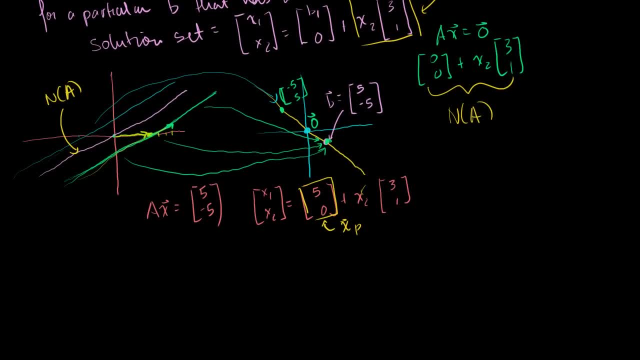 intuition behind it, The solution- and I'll do this in the next video, just because I realize I'm running long on time. Assuming AxB has a solution in the example we just did, we can assume it has if we pick one of these points here. 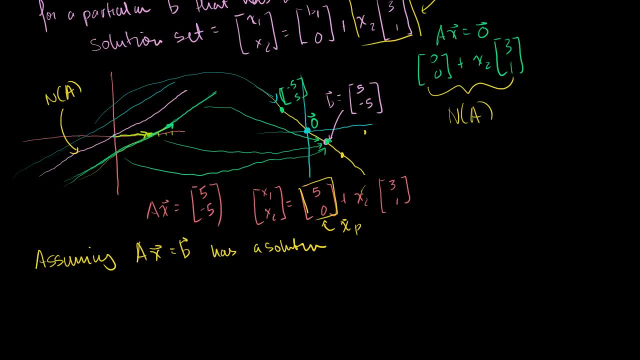 So, assuming it has a solution, if we pick a point off of our image, we're not going to have a solution. But assuming AxB has a solution, the solution set is going to be equal to some particular vector, so you could just think of it as a set with just one vector, right? 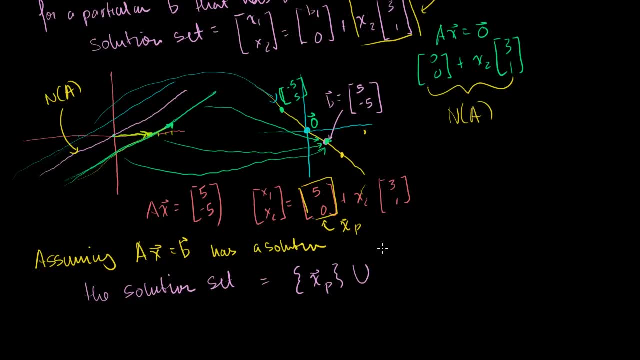 there with, or combined with, or the union of that set with your null space of this matrix right here. I haven't proven this to you yet, but hopefully you get the intuition why this is true. We just solved it for particular cases that do have.